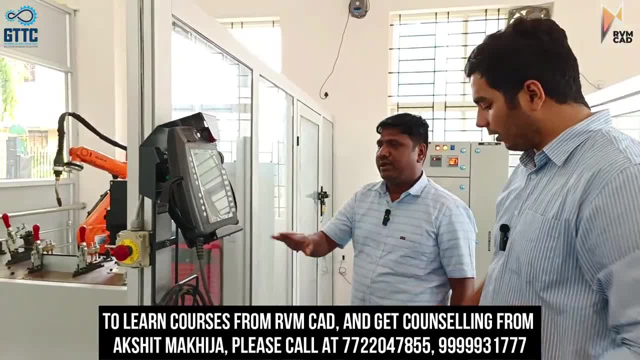 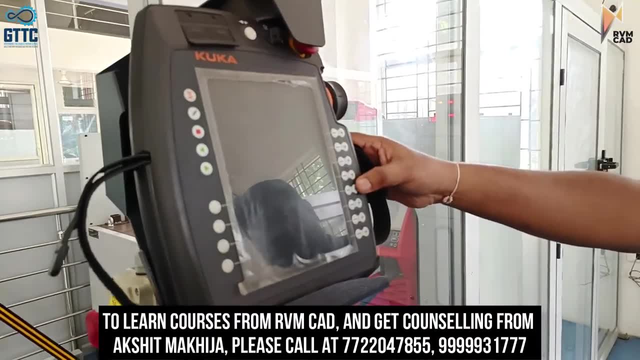 As you can see the smart pad over there. Okay, So you have to basically hold it and then do the programming in this. Okay, So these are all the operation keys. which direction it has to be moved? Okay, Axis one, two, three, four, five. 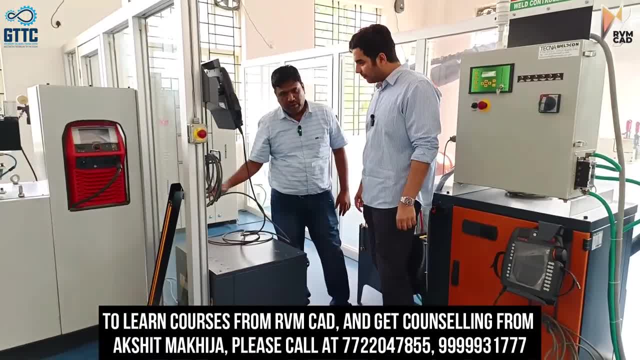 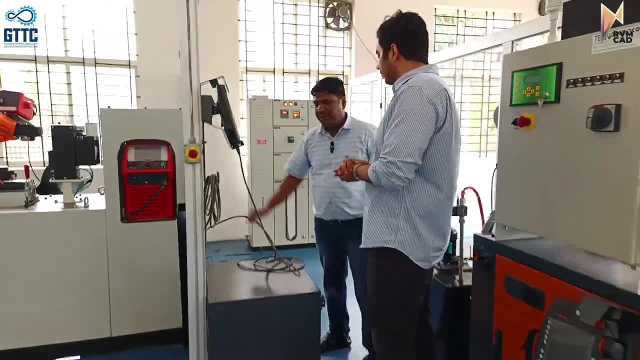 We will see a demo also. Yeah, That I will show later. Yeah, Yeah, CPU of this robotics. Okay, So here it will control from here, So that organ gas is connected to this attachment. Okay, This is a separate attachment that we have made. 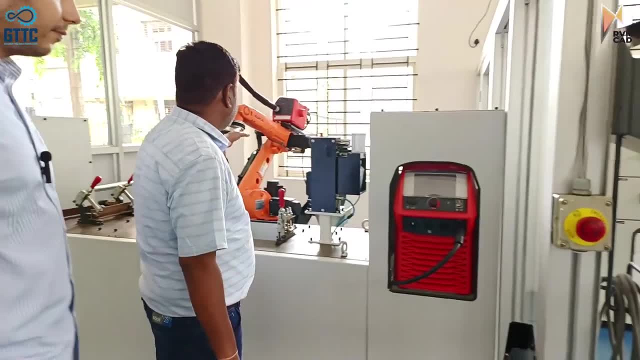 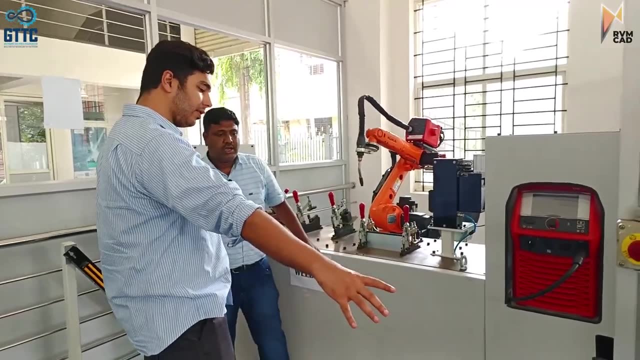 Okay, So this will be synced with that robot. This all thing is about this attachment over there. Yeah, You have mentioned. Okay, So this robot is controlled by this unit And the MIG welding whole setup is separate. Yeah, This one. 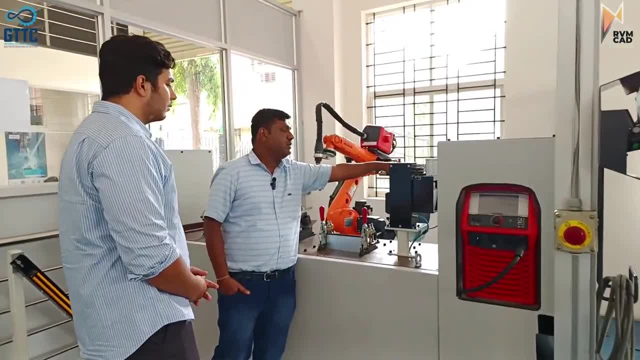 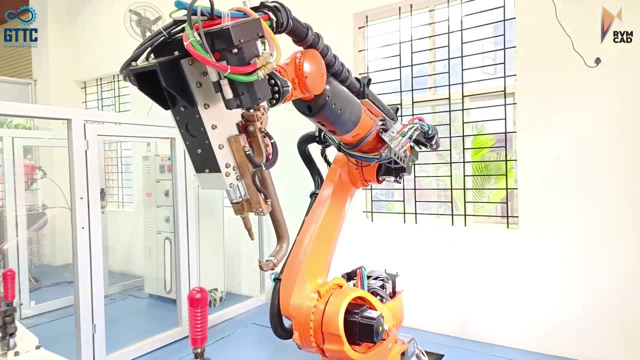 Red color one. This one will operate with to control automatically that how much flow the organ gas has to be done, and these things have to be controlled with this. Okay, That's it. Friction welding like spot welding. What will? the spot welding process is all about doing an high speed friction. 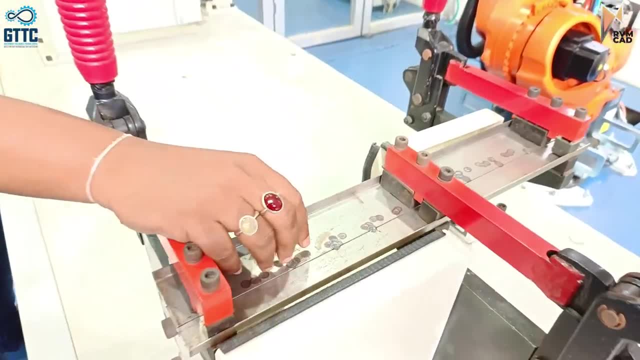 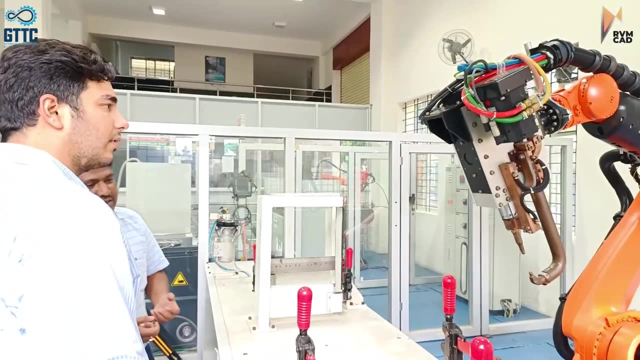 So automatically it will do the welding. All right, Usually we will see these kinds of welding in the busses, like they will do the floor Heavy commercial vehicles. You know, two plates will be joined with the help of friction. Whichever the point I want to fix, 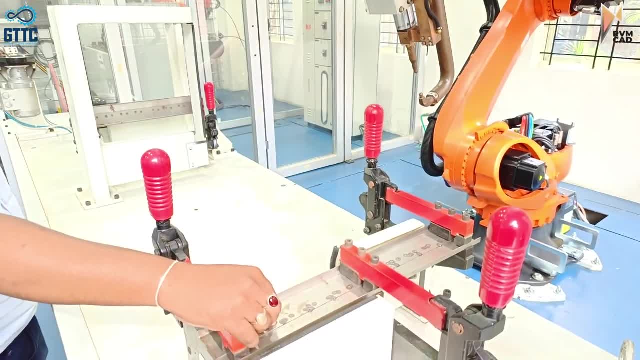 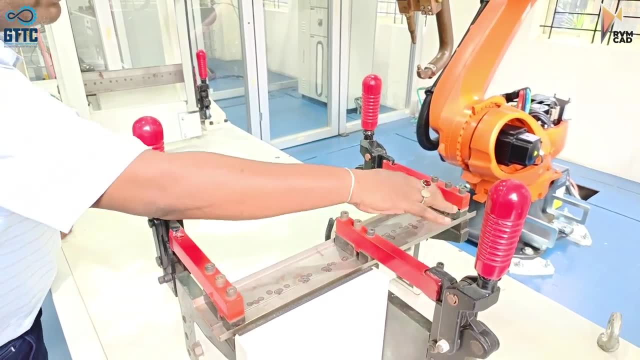 I have to take that robot here and we have to jog and here we have to do the welding Weld operation on and that automatically to do. First we will assign 0.1, 0.2, 0.3, 0.4, 0.5, 0.6, 0.1.. 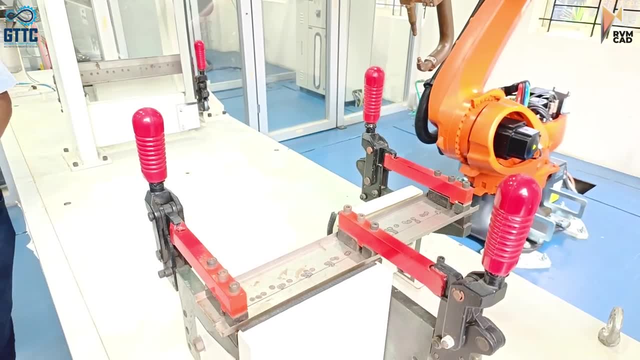 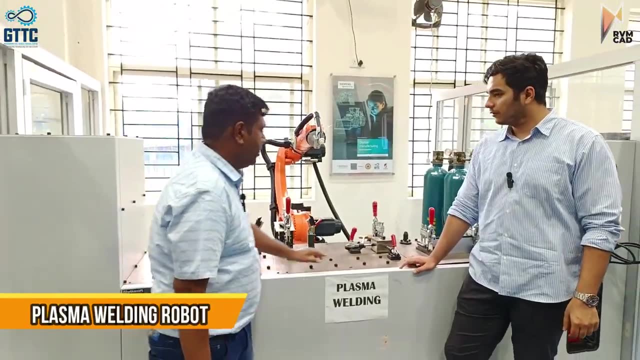 So, similarly, it will do the welding accordingly. Okay, So what about the other robots that we have? No additional materials will be added in this, Only the pure gas welding it has done. So we have to two organ gas lenders over there, Okay. 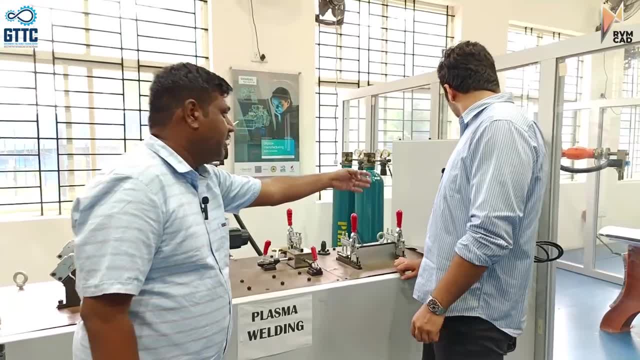 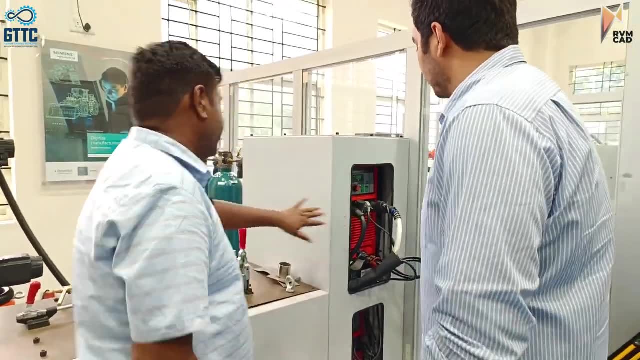 So automatically it will maintain the pressure, Same as we have the additional attachment over there. This will maintain the synchronization. These are all the Fronius things, So Fronius has supplied this attachment. All right To combine the things. This one, KUKA. 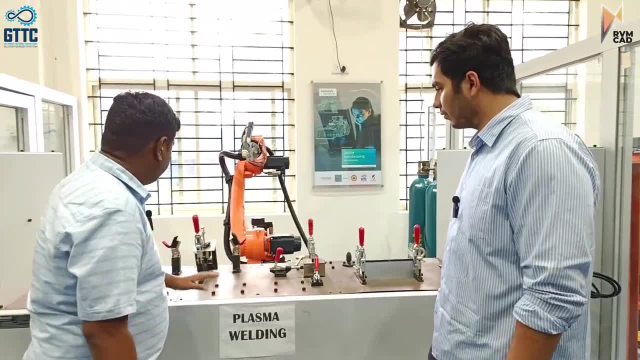 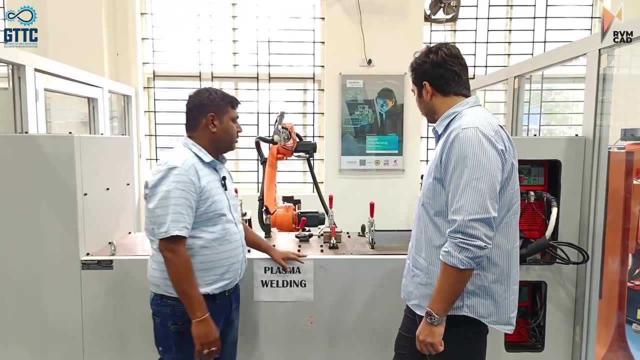 KUKA is a robot and attachment is provided: Fronius. Okay, So these are all the different workstation Like. this one is PEA And this one is circular, This one is a square and this one is butt joint. Okay, 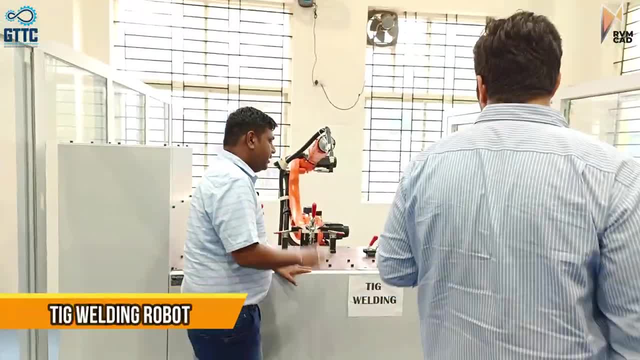 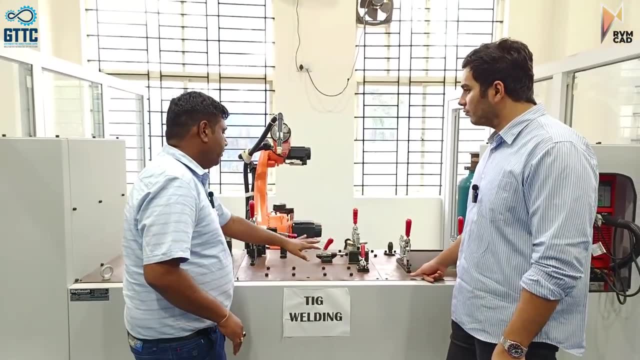 Pure gas welding- this one here. Okay. Tungsten inert gas: Yeah, Same material what we use. total pure gas welding here. The attachment is this one. So it will do electrode based welding, Yeah, With the help of organ gas. 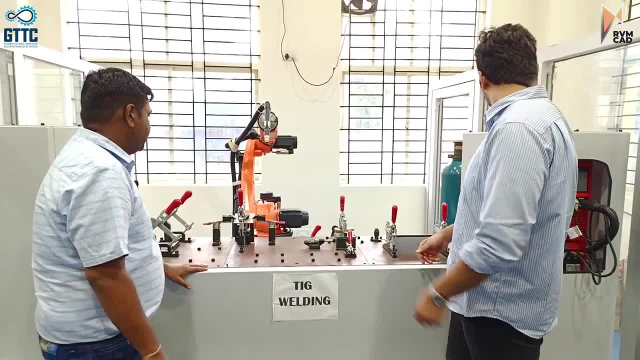 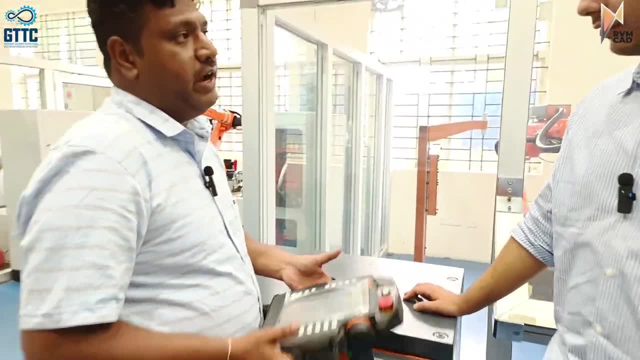 Yeah, So same. this is also attachment with Fronius. only, Okay, All the robots are six axis. Six axis, Okay, Why they provided four means some persons will be left hand, The right hand person, All right, All right. 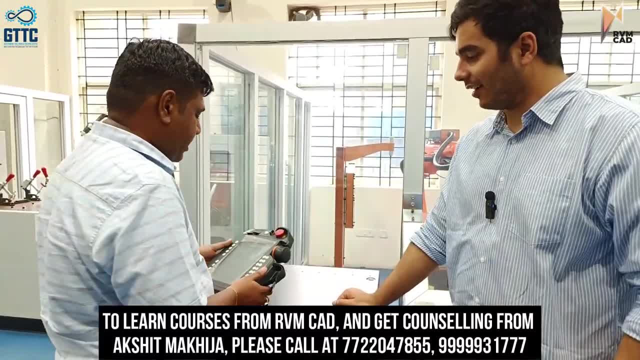 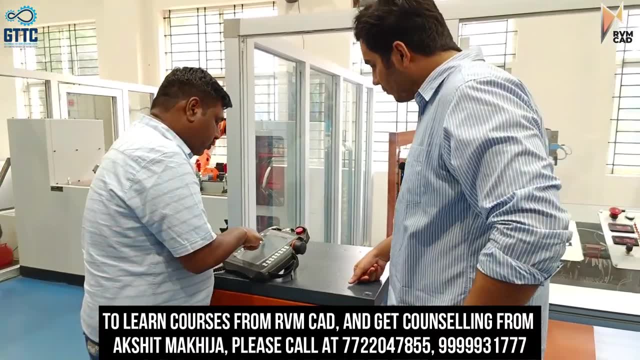 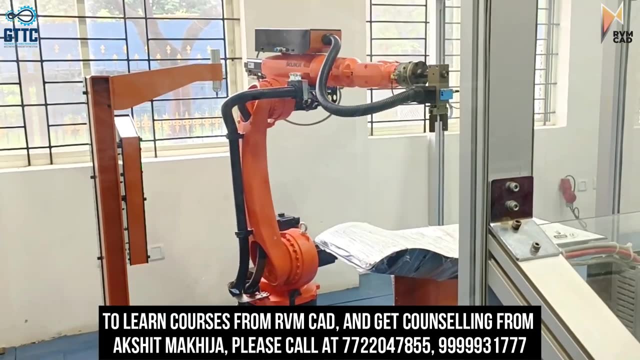 I know this. These are for the brakes. Yes, I know the brakes, Right, Yeah, Yeah, Yeah. Usually we call it enable button. without pressing that, things alone, There are total, Even more people more. automatic, modern auxiliary mode, as I can operate X direction, X, X, minus. 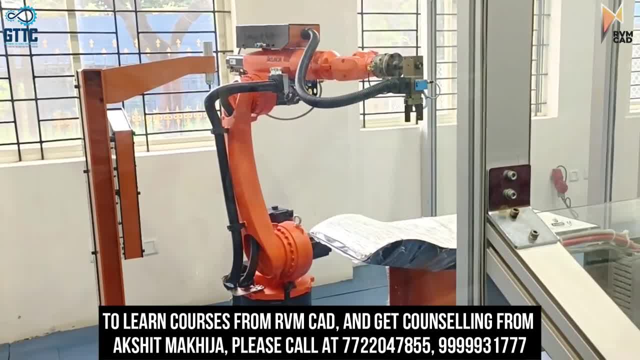 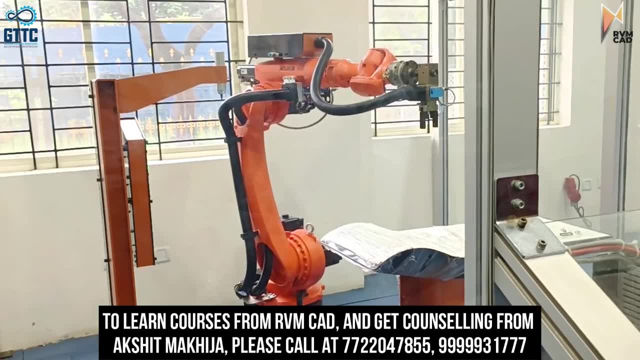 direction, Okay, And it is a positive and negative direction, Yeah, Same. Meanwhile, this is a Y direction. It is going here and here Plus Some, Okay, And this is a job direction up and down. So whatever joints need to be moved to go- X and Y- we will see it on this one. 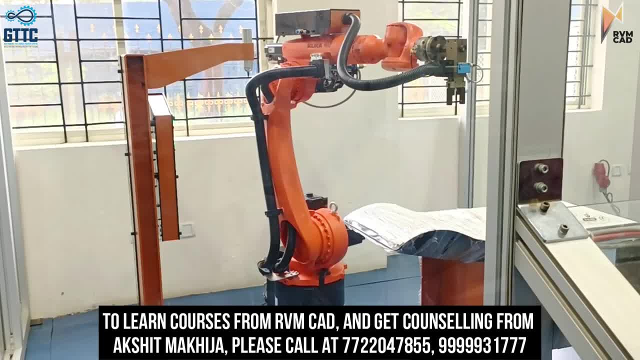 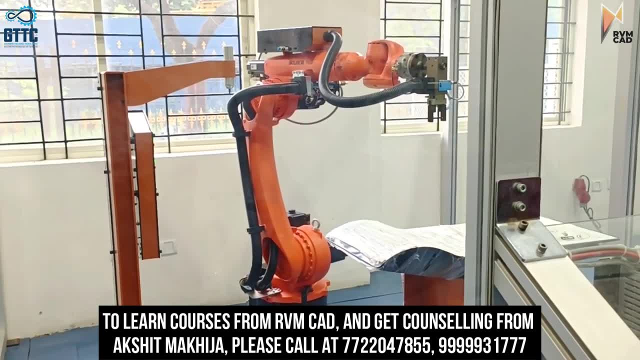 So there are two systems over there. One is this, one is axis based, in axis based. What exactly happens is total six axis are there. Yeah, We will move one by one. We will show which axis are. See first: axis means the bottom bottom plate will move. 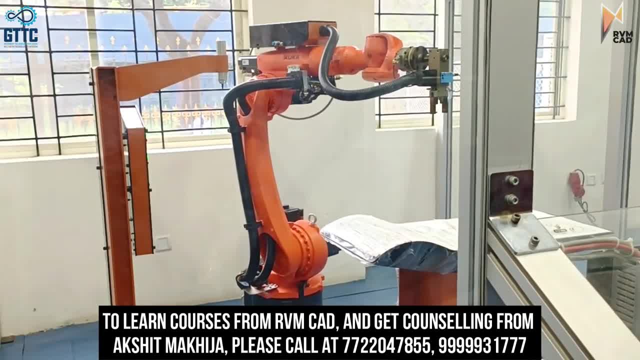 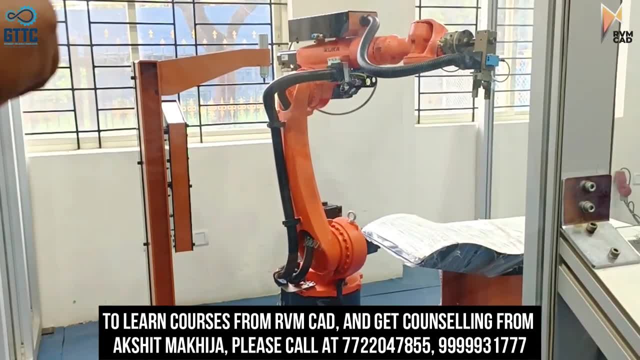 The second one is that. second one. Okay, Only that will move. Okay, Rest of it will be locked, Yeah, Yeah. Third one is that one, and fourth axis is in that direction. Yeah, Already, you can see over there. Yeah. 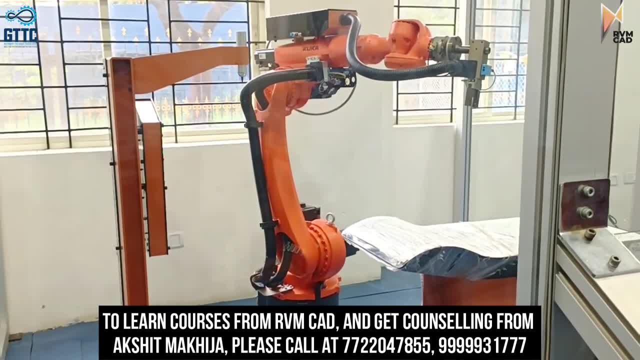 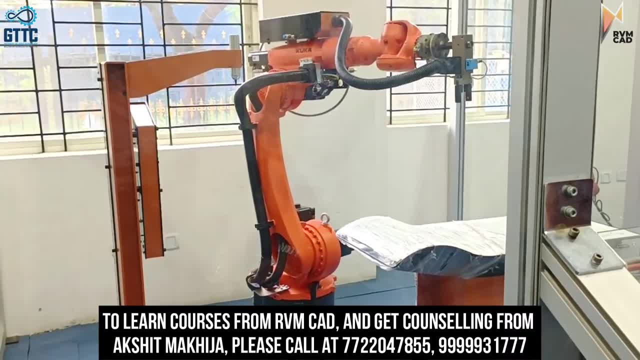 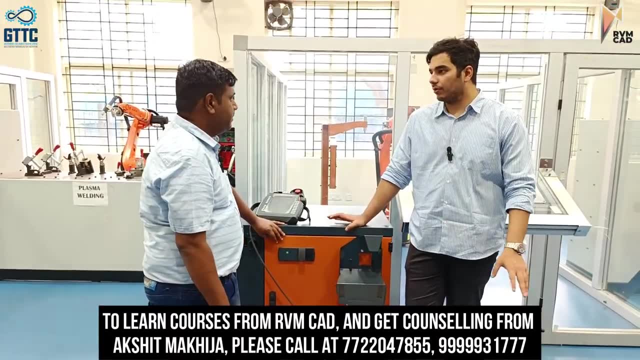 It will be directly attached to that attachment what we have met. Okay, So this is how it works. So, if we have to like teach a student robotics, Yeah, How much time will it take approximately to Yeah, So to know the robotics operation? 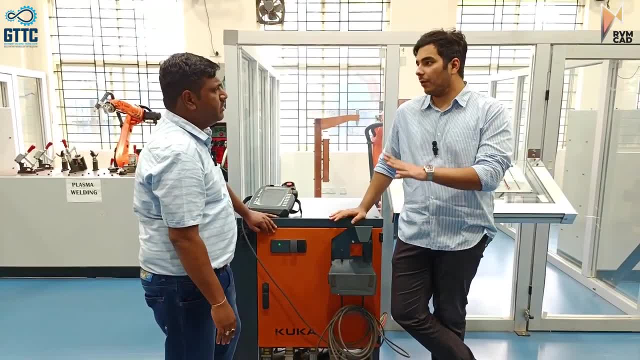 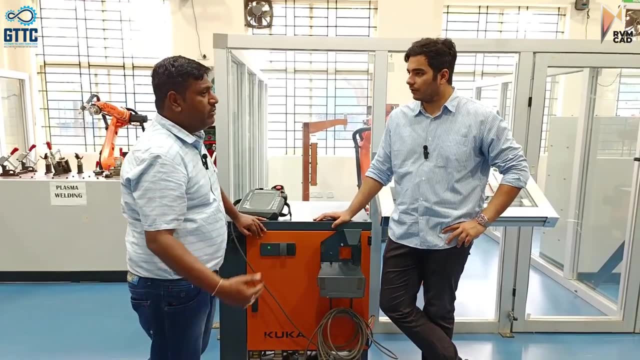 Yeah, How do it will take one, two to three days is how do it will? Basic operation, Not programming, Not programming, Programming and all So programming. what we will do, we will teach them virtual programming. We have one more software backup over there which will help us improve. 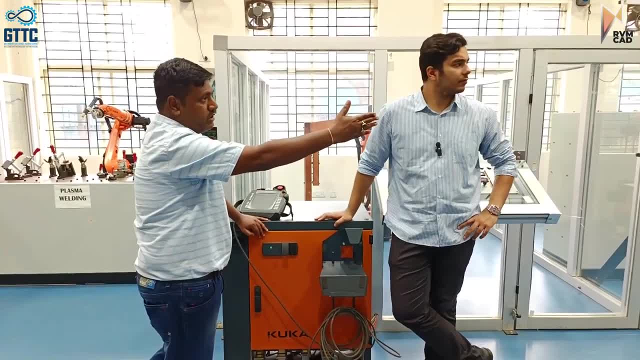 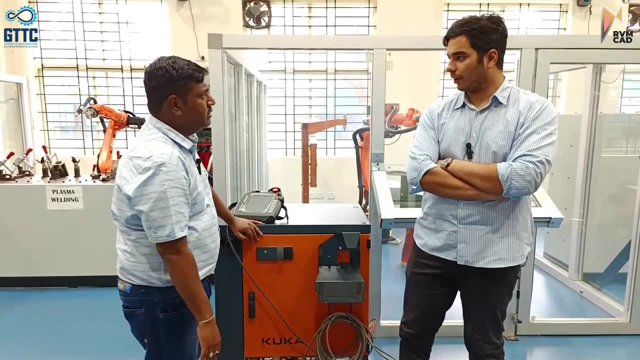 In that we will virtually teach them as we have already wrote the programs over there. That is point to point, and linear and auxiliary Auxiliary is nothing but circular thing. So to become a professional it should take at least 15-20 days of practice. 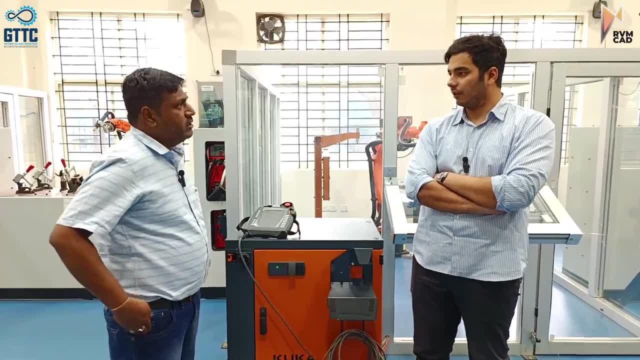 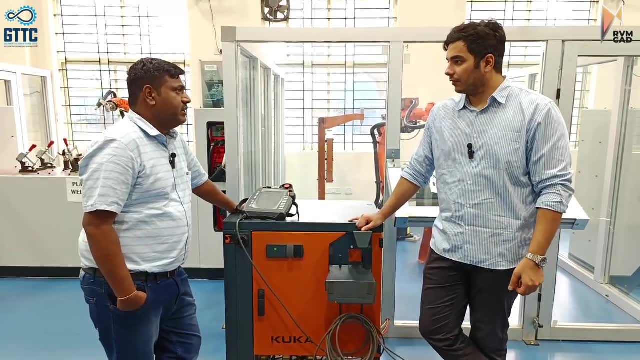 Yeah, 15 days is the standard, sir. 15 days is the standard duration, sir. What are the career options? As we know, all industries are moving to latest technologies. Nowadays this is the fourth generation. In every industry they are using robots. 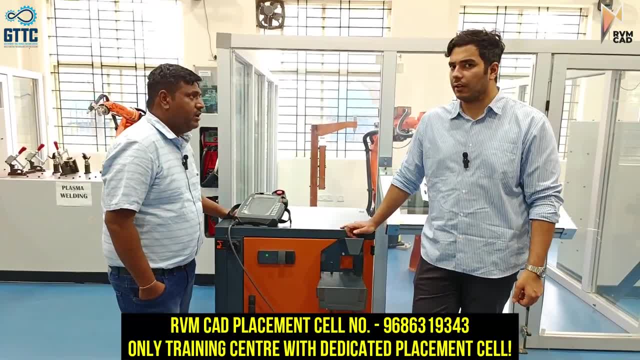 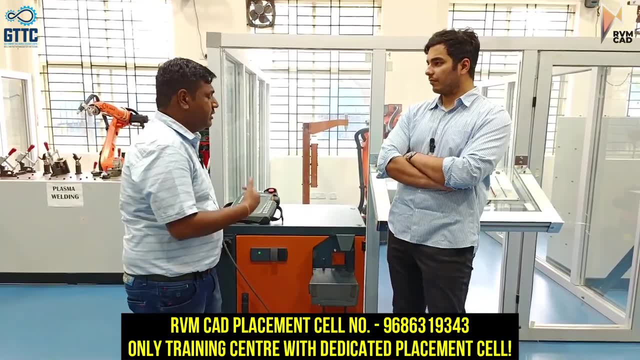 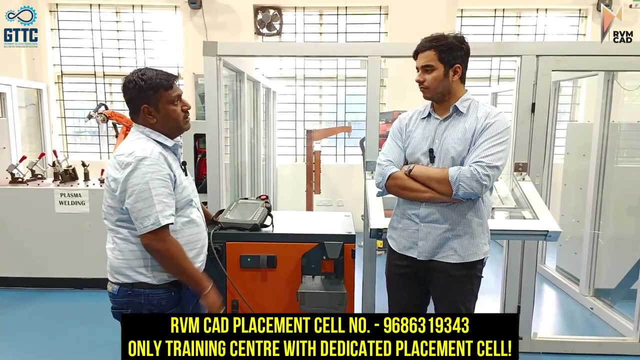 So if you know the programming and operating, so it will always very much add on experience to them. And again, these are all automation things. Before coming to this, if you have a basic knowledge of PLC, that will be very good. That is very good. 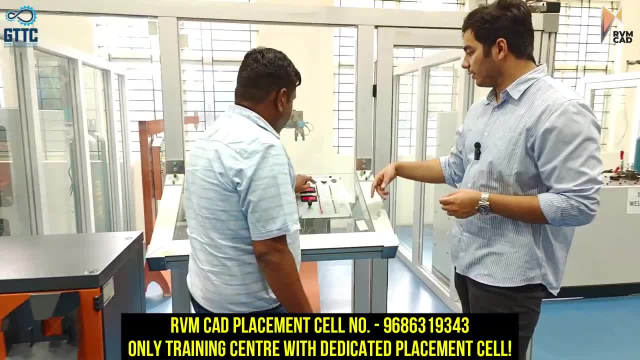 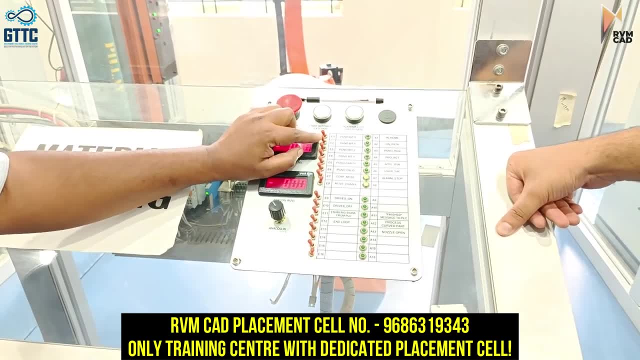 As you can see, Yeah, These are all the PLC connections. PLC is different. 1,, 2,, 3 and 4, we already only 4. we have made auto program, Yeah. So if you want to take permutation combination for program 1, program 2, as you can see over here, these are all plenty of programs. 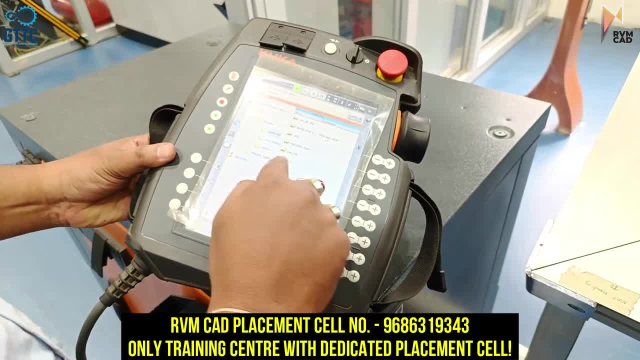 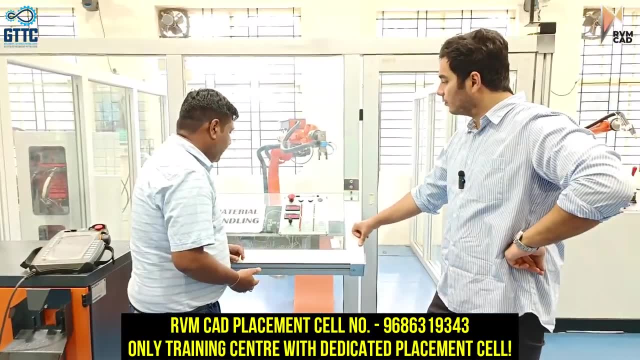 It is block pick and place circular pad. pick and place pad test pen 1,, pen 2, pen 3.. So these are all the programs we have defaultly added over here. Okay, So if you want more program to be done, so we need to have a knowledge of PLC too. 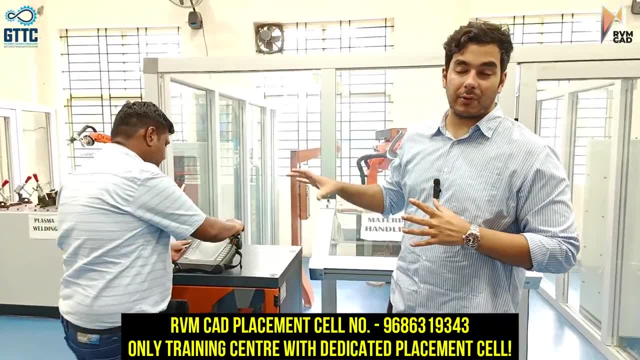 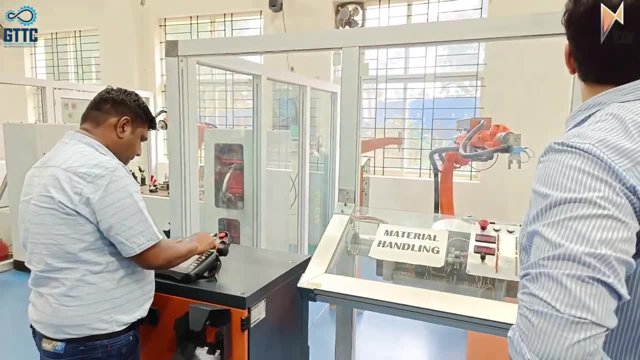 Yes, So we will run. like see a sample of the program in which it will run on its automatic way. Yeah, So we can see now. So why is it showing this kind of noise? It is emergency alarm, I think, Huh. 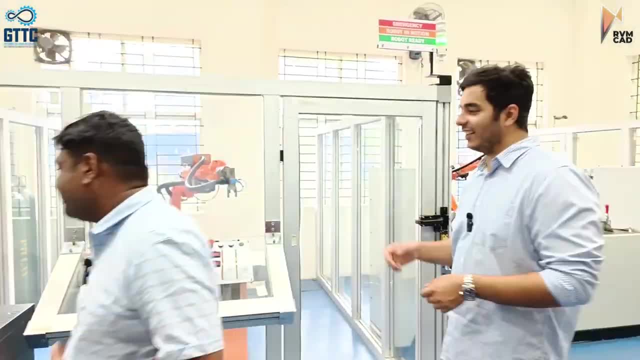 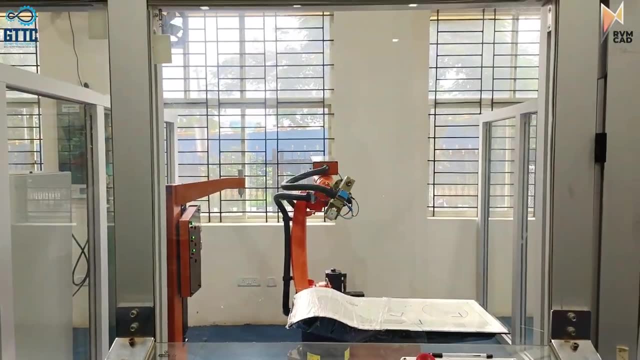 Maybe They are not blocked, So it's safety is very important. So this is a sensor safety. Yeah, That's, Yeah, Okay, Wow, It's picking up. The basic result of the robot is it has to perform an automatic program only. 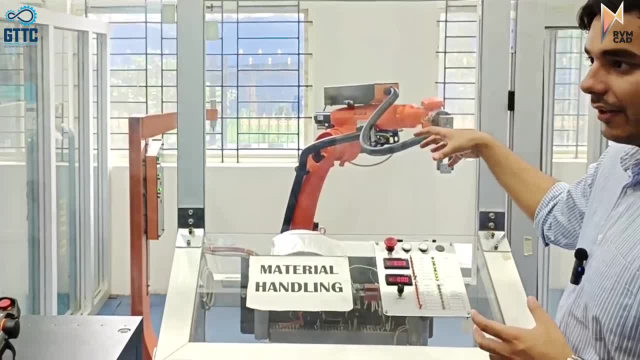 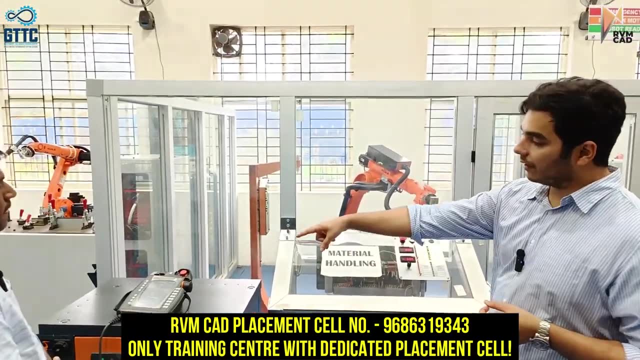 Okay, So there is a cube. it will place it directly on that. Yeah, it will do. Okay, Wow, Just Yeah, Perfectly aligned. Yeah, So it's running from this code, which is already loaded into this. Yeah. 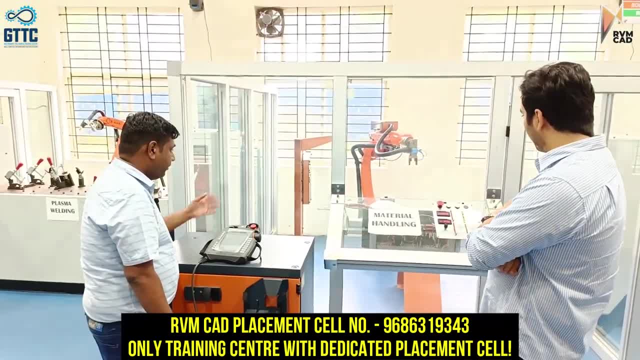 It is already. We have already mentioned the code No. Okay, Here it will say: wait After keeping that we have to wait for 5 seconds And then Then again it will take there and it will dump back again in that position.